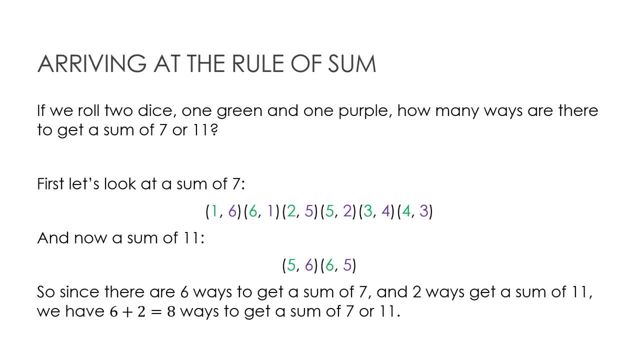 to the correct solution. So instead of just providing you with the rule of sum, let's talk about how we might arrive there. I have two dice, one green, one purple. How many ways are there to get a sum of seven or 11?? So typically what students do, starting out, is say: 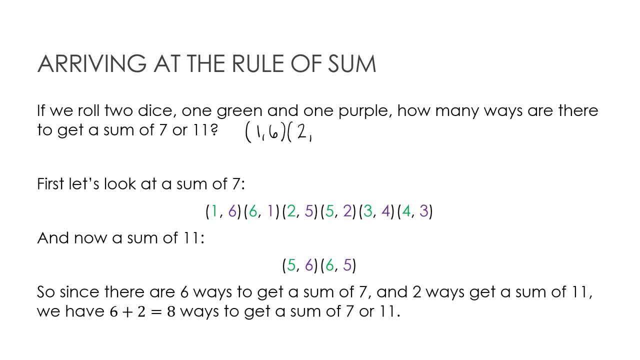 I could get a seven with one, six, two, five or three, four, And I could get an 11 with five, six, And so they'd say there are four ways, But, as we can see, it's not quite as simple as that. 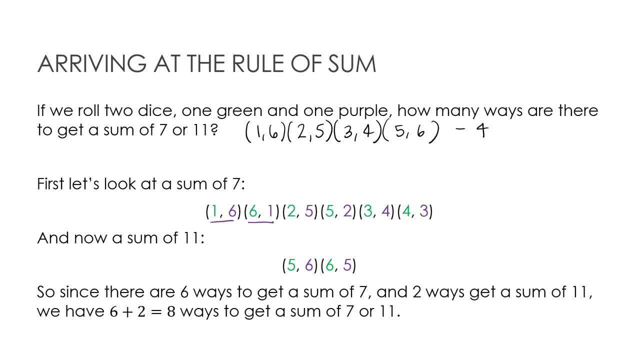 because one six and six one, even though they are kind of the same. I'm rolling one one and one six and I've color coded them so you can see which die was which color. One, six and six one should both be options for us. Two, five and five. two should both be options for us. Three, four and. 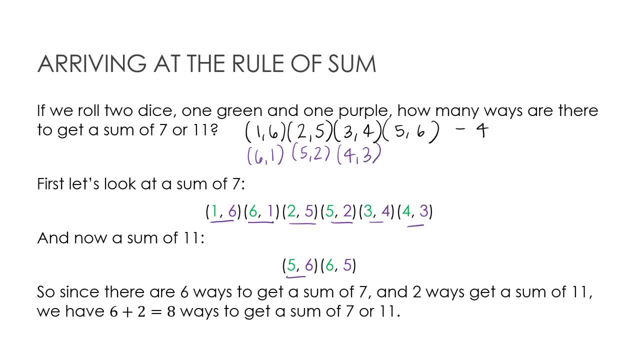 four, three should both be options for us, And then five, six and six, five should both be options for us. So how many ways are there to get a sum of seven or 11?? Well, there are six ways and two ways, So there are a total of eight ways. So this brings us to the rule of sum. The rule of sum. 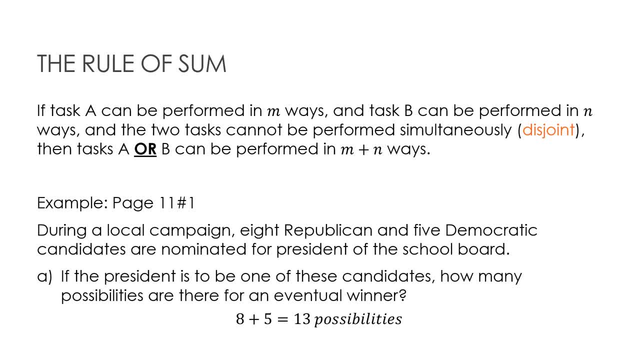 states that if I have two tasks, one which can be performed in m ways and one in n ways, and the two tasks cannot be performed simultaneously, which means they are disjoint, which is essentially saying, when I roll, I can't get both a sum of seven and 11 at the same time. 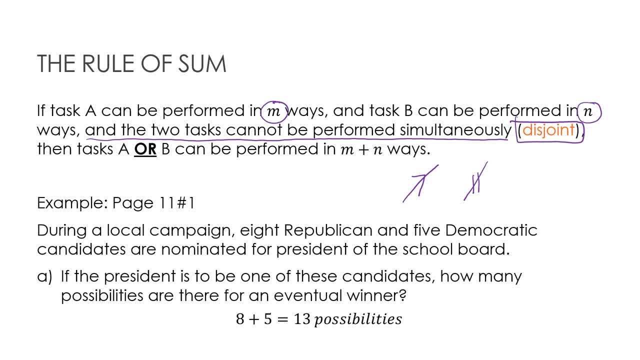 I could get a sum of seven, or I could get a sum of 11.. Then test A or B can be performed in m plus seven. So I can get a sum of seven, or I could get a sum of 11.. Then test A or B can be performed in m plus seven, or I could get a sum of 11.. 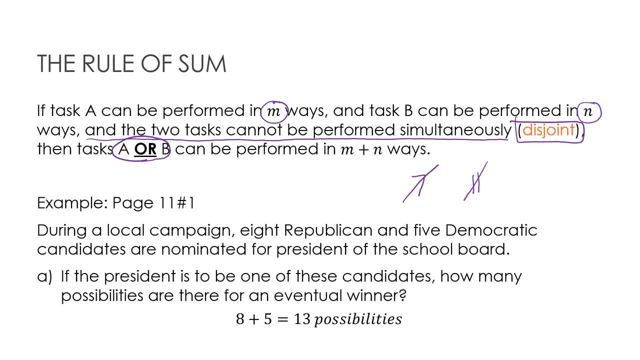 So there are six ways and ways. So what I want you to start to associate is when you see something that's or you should be thinking plus. So if I'm saying A or B, I'm going to be adding those possibilities together. Here's an example. This is from your textbook, page 11, number one. 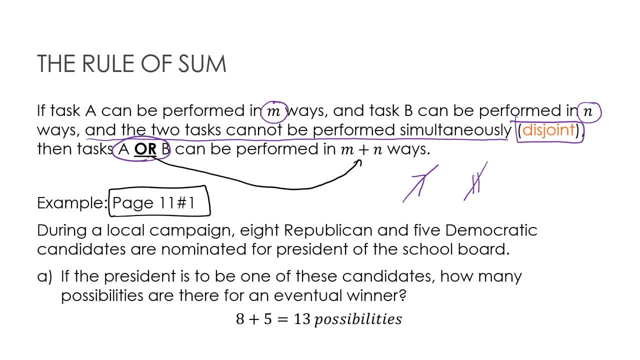 During a local campaign, eight Republican, five Democratic candidates are nominated for president of the school board. If the president is to be one of these candidates, how many possible candidates are nominated for president of the school board If the president is to be one of? 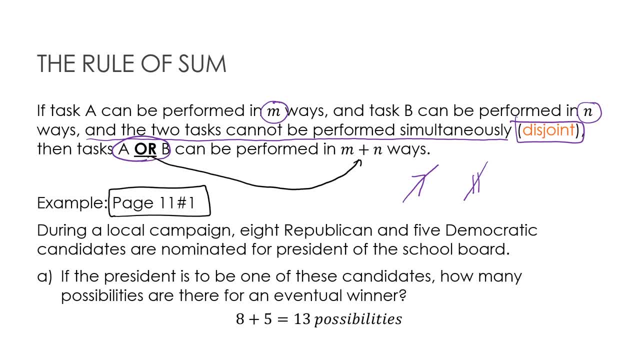 these candidates, how many possibilities are there for an eventual winner? Well, again, this is very straightforward: There's eight Republicans, there's five Democrats. One of them is going to end up being president of the school board, So let's just add those together to get our 13. 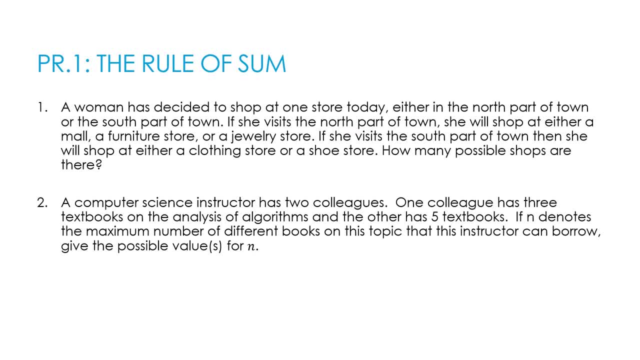 possibilities. So quite often, what I will do is provide some practice questions which go above and beyond the examples that we go through together. So whenever you see one of these PR1, PR2, etc. those are going to be the ones that you're going to want to practice. So I'm going to practice that if we were. 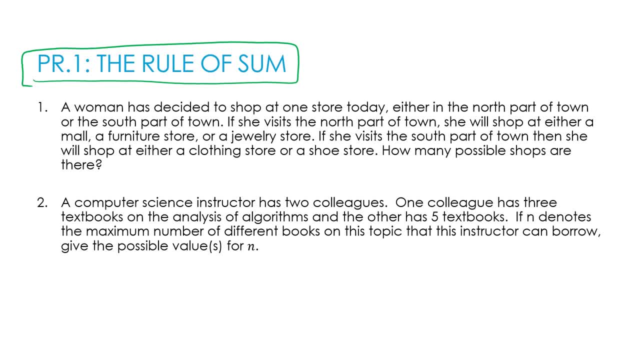 sitting in a classroom together. I would ask you to turn to your partner and work together to solve these two, or possibly solve them on your own, Since you're watching this video instead of being in a classroom with me. what I'd like you to do every time you see one of these is to press pause, take. 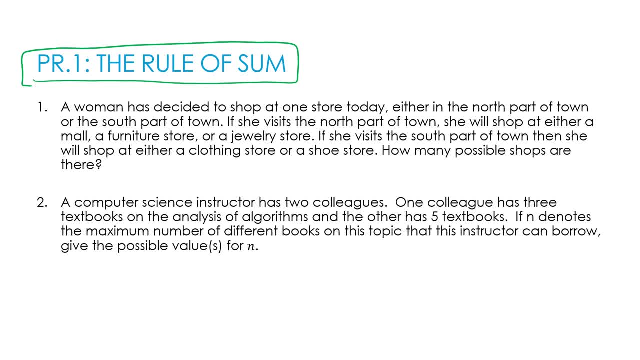 your time as you would in a classroom, to read each question, to try each question and then, when you are ready, I would like you to press play to see how you did. So hopefully you did actually press pause and try these questions and you're not just waiting for me. 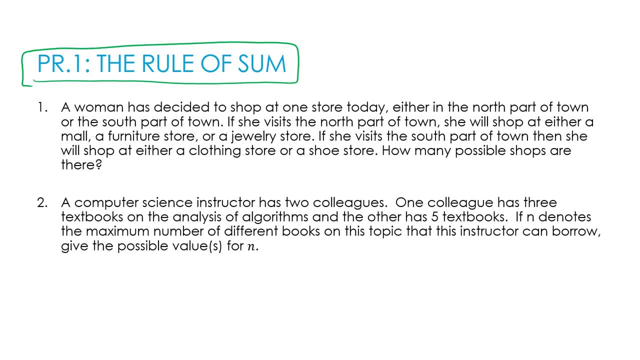 to go over them. Question one: we're looking at a woman who's deciding to go shopping and she's either going to go north or south, And if she goes north, she's going to visit a mall, a furniture store or a jewelry store. So going north provides us with three options. If she goes south, she's. 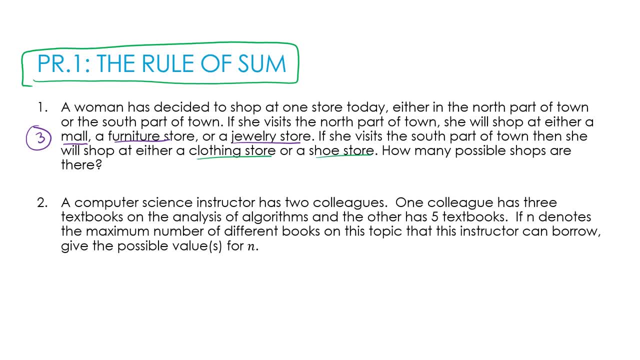 going to shop at a clothing store or a shoe store. So going south provides us two options. This is a very straight up rule of some question. All I have to do is add the two together. Three plus two equals five possible shops that she could go to, And again, that's answering the question that was. 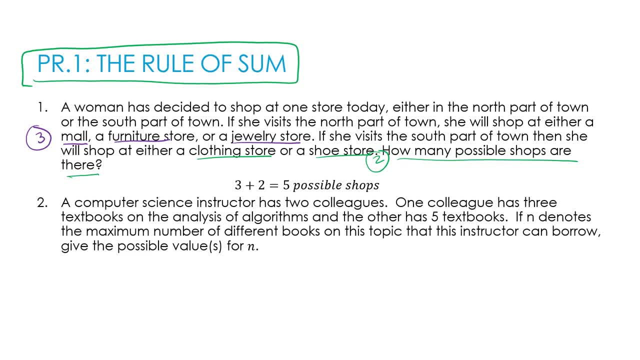 asked Question two, not quite as straightforward. This one says a computer science instructor has two colleagues. One has three textbooks on the analysis of algorithms- Great reading, I'm sure- And the other has five textbooks- The maximum number of different books on the topic that the instructor can borrow. 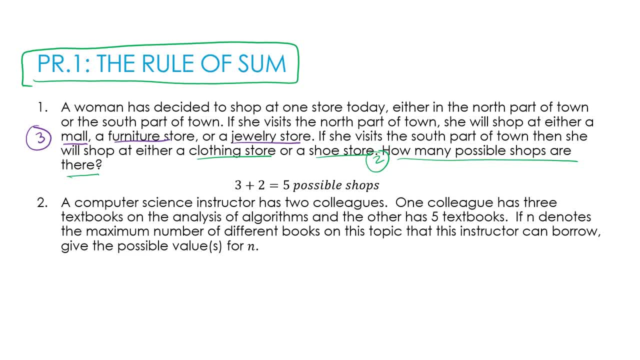 give the possible values for n. So key word here that I want to point out is that we're talking about different books, So a lot of people would just say, well, if one has three and one has five, that means there's eight. And you're partially correct. There are eight possible. 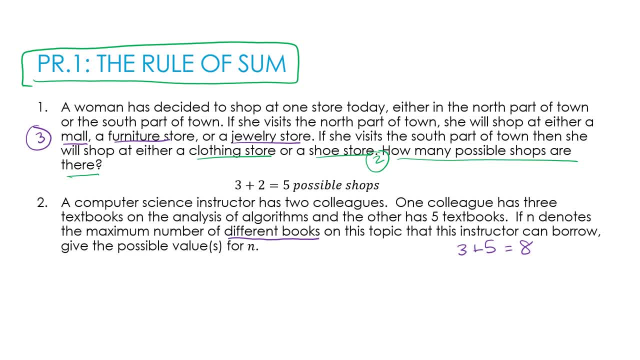 textbooks that I can borrow from my colleagues. However, because I'm looking specifically for different books and it doesn't specify if the first colleague and the second colleague have different textbooks, it could be that all three of my first colleague's textbooks are also in my second. 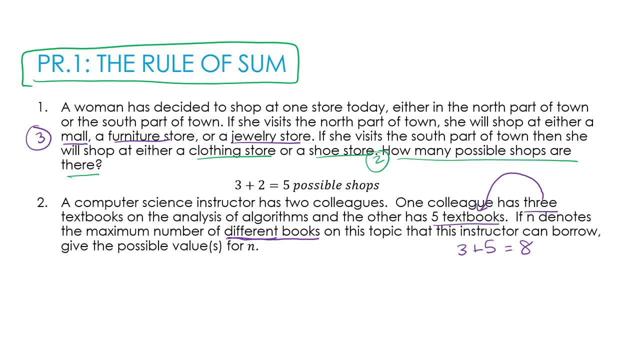 colleague's textbook library. So what I'm going to do instead is say that there are up to eight. three plus five does equal eight, just as we said before. But it's possible that there is an overlap of one, two or three of those textbooks to be the same. So that way you'reформating the answer on the. 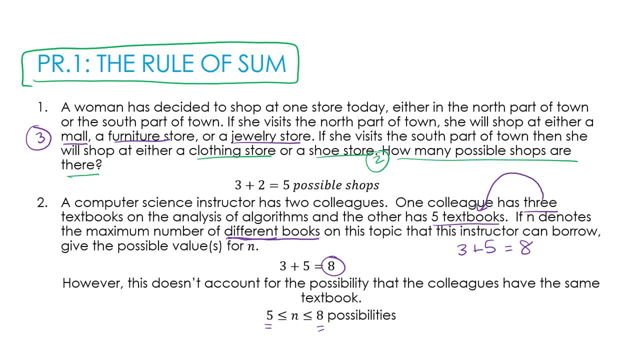 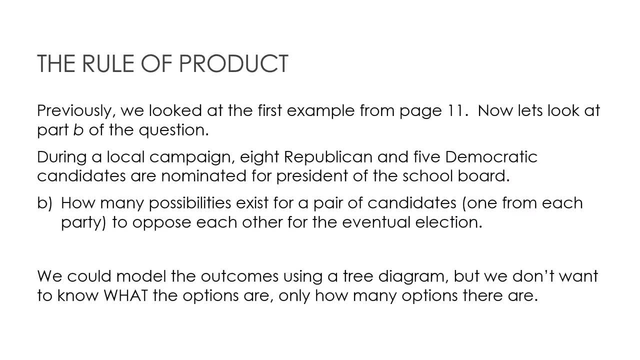 So it's possible that only the five that I get from my second colleague will have five different textbooks, So anywhere from five to eight inclusive. So previously we looked at example 1A, which was in your textbook on page 11.. Now I want to look at part B of that same question, because I want to talk about the rule of product. 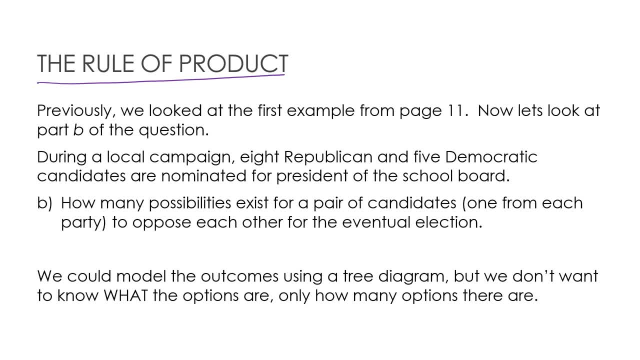 So, during a local campaign, eight Republicans and five Democrat candidates are nominated for president of the school board. This question is different: How many possibilities exist for a pair of candidates, one from each party, to oppose each other for the eventual election? Now, obviously, there's a very simple way to do this: using the rule of product. 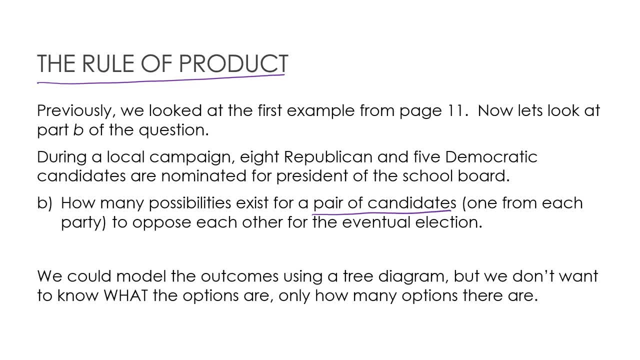 If we didn't have the rule of product, you might have to make a tree diagram. So a tree diagram, in case you don't know, is something where I would put my eight candidates that are Republican: One, two, three, four, five, six, seven, eight. 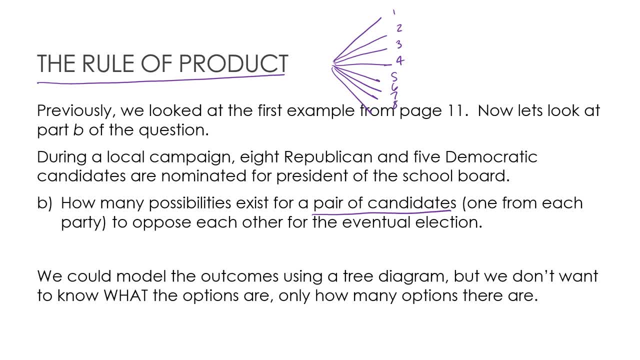 And off of each of those eight, I would pair them with each of the five Democratic candidates. So each of these would have five branches- and I'm not going to draw those branches- And that would be the one, two, three, four, five candidates for Democrats. 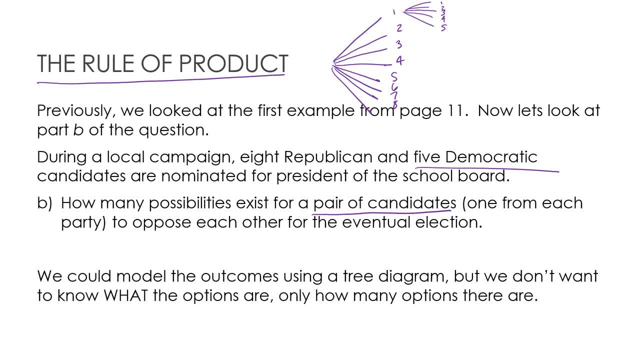 So if I needed to know all of the different possible combinations, I would have to make a tree diagram. but what I'm looking for are just how many options are there? So if I don't care about what the actual combinations are and just need to know the number, 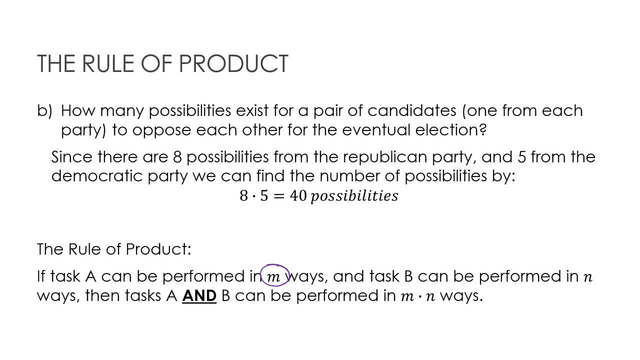 I'm going to use the rule of product, which looks similar to what we've said before, for rule of sum. If one is m-ways, one is n-ways. Notice, if it's a and b, then I'm going to multiply. 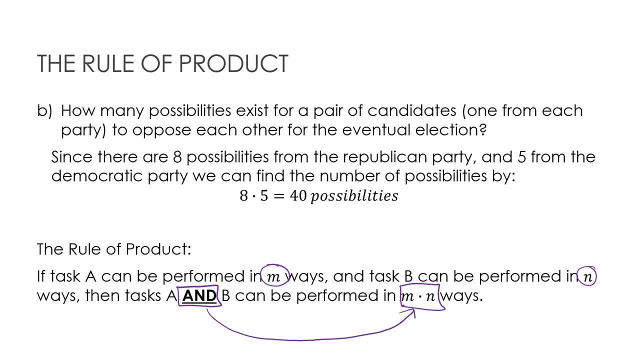 So again, you should start to associate, and with multiplication. So, going back to our question, there are eight possibilities from the Republican Party and five from the Democratic Party. The number of possibilities is found by taking eight times five, because I'm using one Republican and one Democrat. 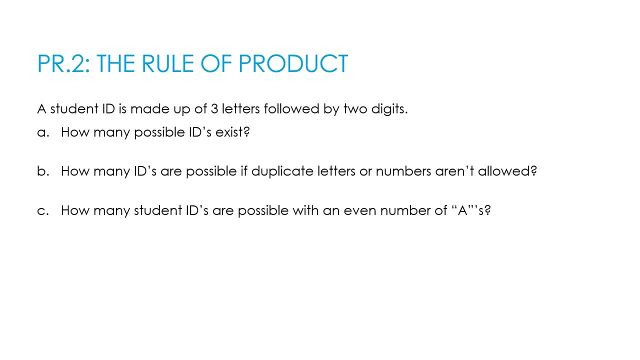 So I get 40 total possibilities. So here's another practice for you, And again, some of these will be very straightforward and some not so much. So what I want you to do is press pause, try all three questions, then press play to see how you did. 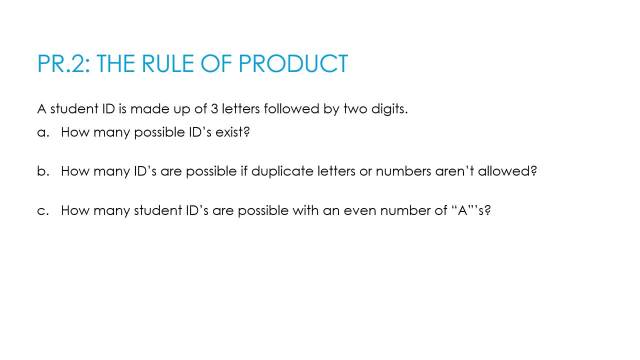 So I'm starting by looking at a student ID made up of three letters followed by two digits, and it says how many possible IDs exist. So, starting to look at this, I would say there's three letters and two digits. So letter, letter, letter, digit, digit. 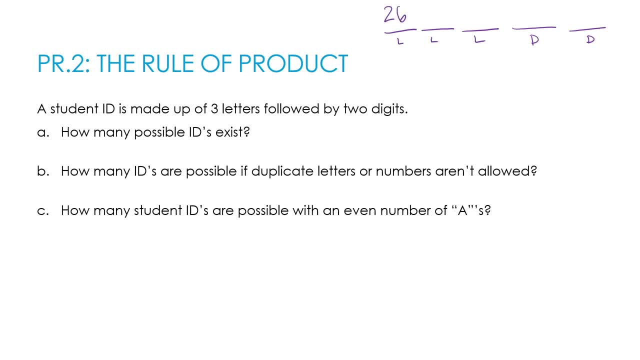 Well, how many letters are there? There's 26. And there's no restriction right now. It doesn't say I can't repeat letters, So there's 26, three times And two digits. Digits are the numbers zero through nine, which means that there are 10 digits. 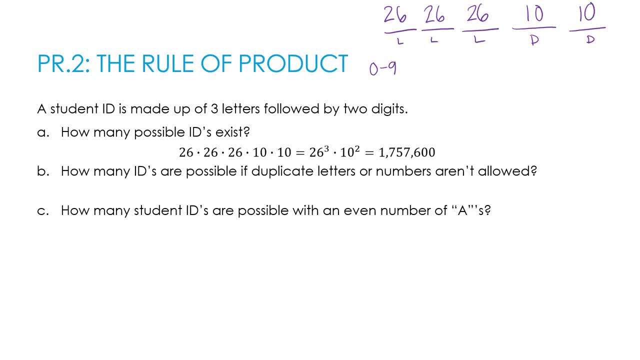 So that's going to be my first solution. Twenty six to the third times 10 squared and multiply it out Now in terms of answer format. if you're able to show me both how you set it up and the solution, that's great. 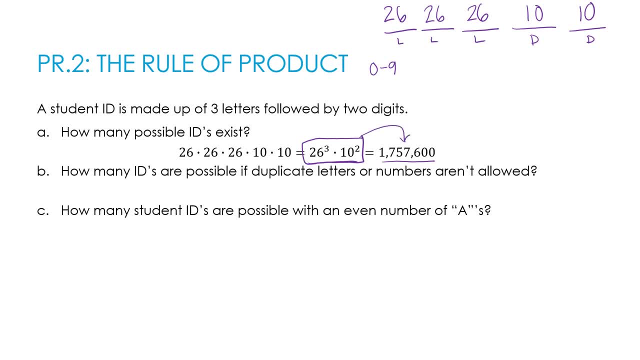 Sometimes, especially later on in the course, we're going to have numbers that are so large that this is going to be the answer, So I'm going to go ahead and do that. This will be your final solution and you won't have to multiply it out. 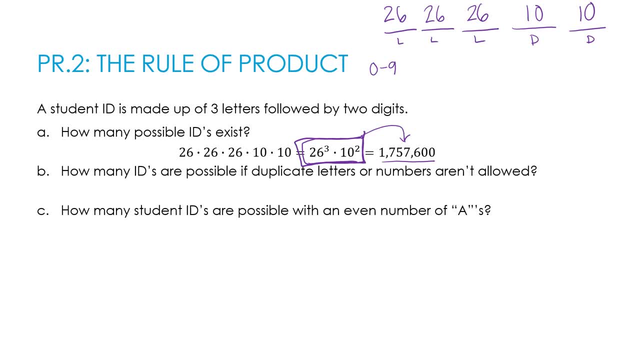 But for now please show me both. For B, it says how many IDs are possible if duplicate letters or numbers aren't allowed. So let's take a look at how my little display at the top might change. If I have 26 letters for my first option, then my second option is now 25 letters, because I can't use whatever letter I used here. 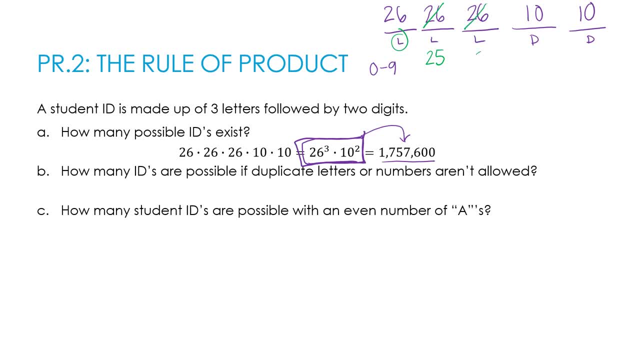 And then my third letter. I only have 24 options because I can't use whatever letter was second or first For my digits. I've got one digit that can be anything, that I want it to be 10.. But my next digit has to be anything except for what I chose here. 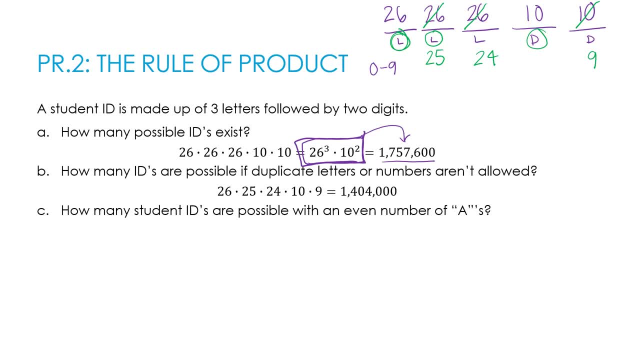 So that's going to be my new solution: Twenty six times 25 times 24 times 10 times nine. And again I choose, And again I found that as a raw score as well. Last one: this one's a little bit tougher. 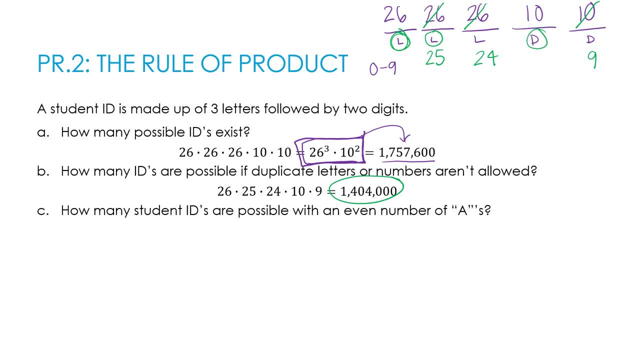 How many student IDs are possible with an even number of A's? So first, we need to think about the fact that we have three letters, so it's possible to have zero A's And it's possible to have two A's, But, just like we talked about before, where one six and six one should both be options. 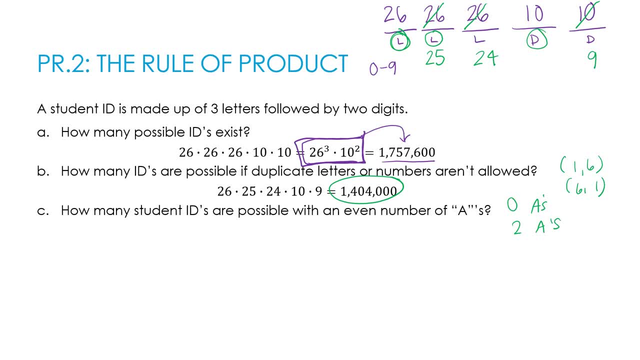 We have different possibilities for where those A's will go. So let's take a look at how I broke this down, And quite often you'll see your work like this. Here are my three different ways that I could have two A's, So I could have AA and then some other letter. 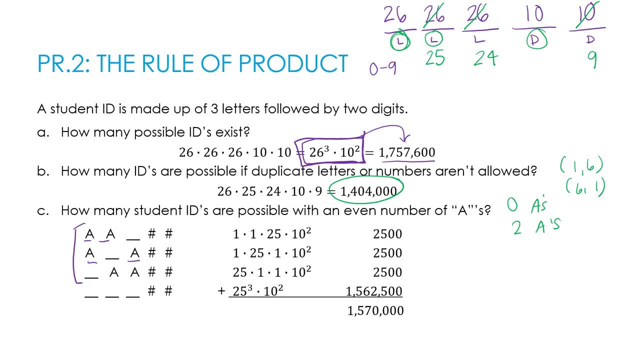 A, some other letter A or some other letter than AA. So those are all the different ways that those could happen, And then whatever number I have here and here. So what do those look like? Those are all: one option for the A's and 25 options, which is every letter except for A. for the other space, 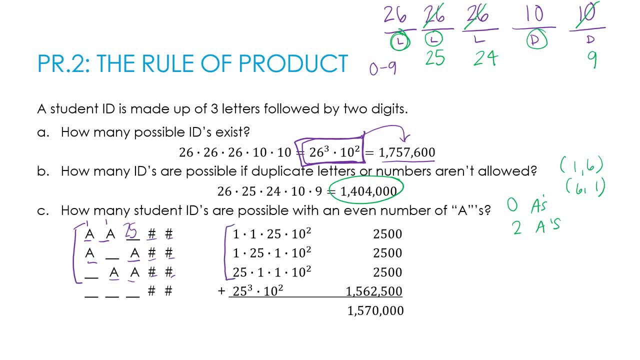 So, if you'll notice, the three of these are exactly the same. I put the 25 in a different place to signify where the blank was, But really this is just three of the exact same thing. For the last one, for zero A's. 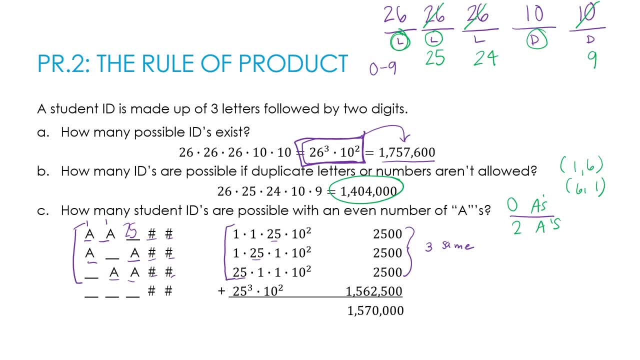 I know that there are 25 options, which means not anything but an A, anything but an A, anything but an A, And then, of course, 10 squared. Then all I did add all of those up to get my final solution. 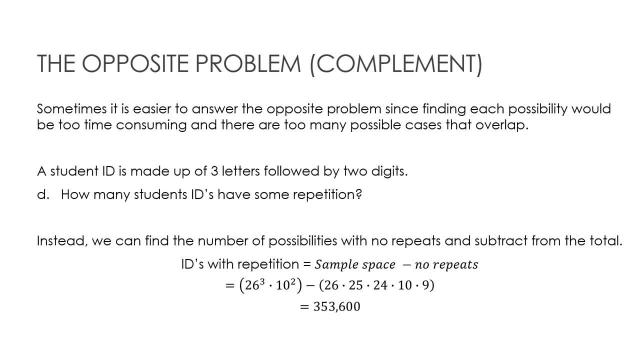 Let's take a look at our last concept for section 1.1, which is the opposite problem, also known as the complement. Now, you should be familiar with the word complement. Previously, when we learned about probabilities, we would say the probability of not A would be 1 minus the probability of A, or vice versa. 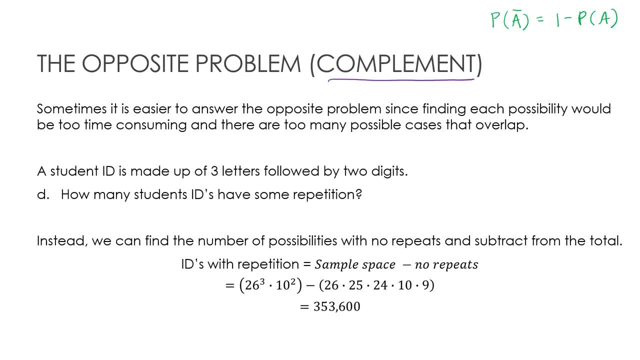 That's what the complement is all about. Now, when we did this with probabilities, we used 1, because 1 was all of the probabilities put together, Because we know that a full sample space needs to be 1.. So let's take that same concept and apply it instead of probabilities. 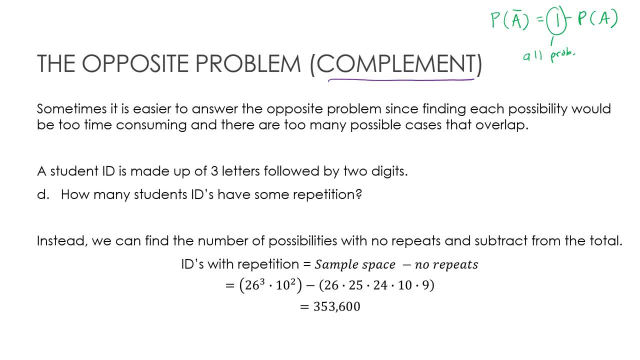 Let's apply it now to A. Let's apply it now to the number of options that can occur. The part D of the same question that we were just working on with student IDs says how many student IDs have some repetition, Which means, if I were going to do this without the complement, that we haven't learned yet. 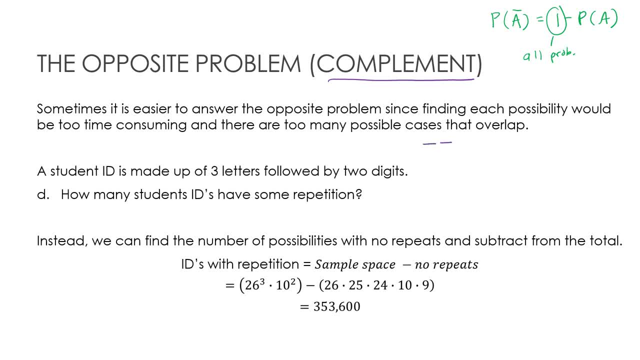 I would have to find what happens if I had two A's here and then some other number and two B's And some other number and two C's and some other number, And then I would have to put the A's here and here. 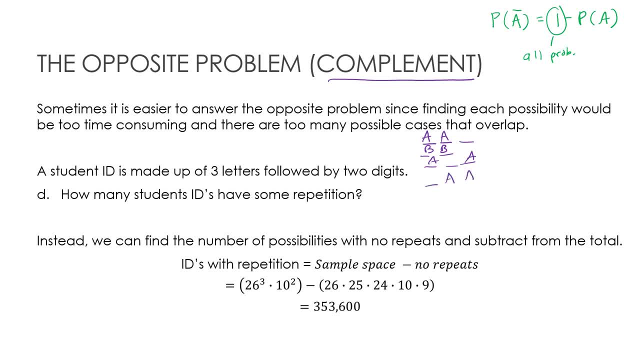 And then I would have to put the A's here and here, And then I would have to put the A's all over, And then B, B, B and C, C, C, And I haven't even looked at the numbers yet. 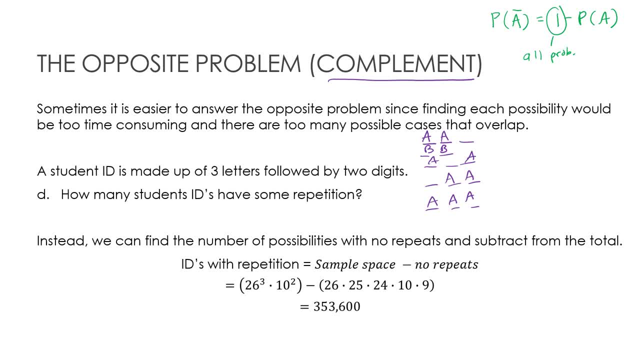 So you can see that if I was trying to do this using the rule of sum, there would be just so many options that I would have to find, And it's very possible that I would screw up and forget one. So instead of doing that, because that would be ridiculous, 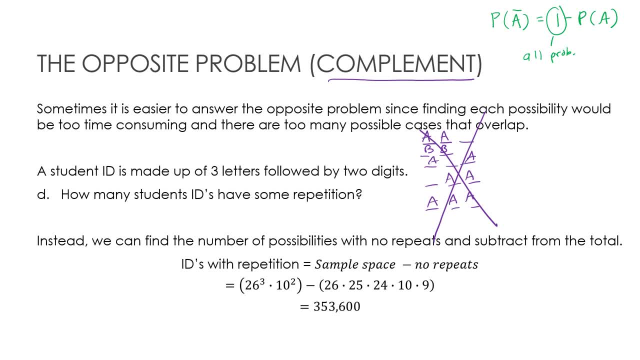 let's take a look at the complement. The complement of having some repetition would be no repetition. So if I can find how many where there are no repeats, no repetition, and subtract it from the total like I did up here, but the total won't be one. 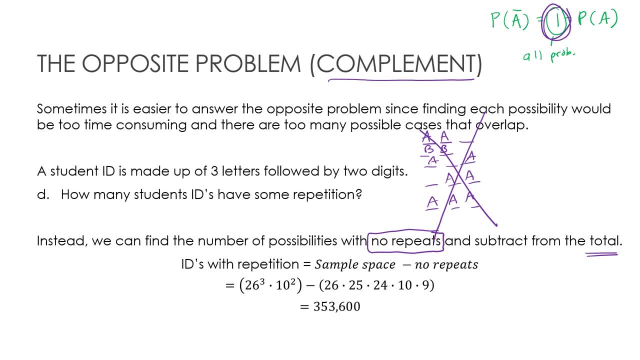 it will be the total number of options. then I'm in business. That's how we use the complement. So let's take a look at how I might do that If I were looking for the total sample space. well, we already kind of figured that out. 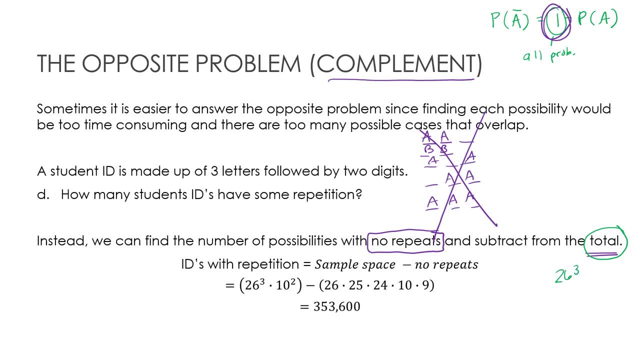 We said that there were 26. to the third times 10 squared because there were three letters and two digits. So that's what I have here. That is ID's total sample space. The no repeats is obviously a little bit harder. So I'm going to say there are 26 options for my first letter. 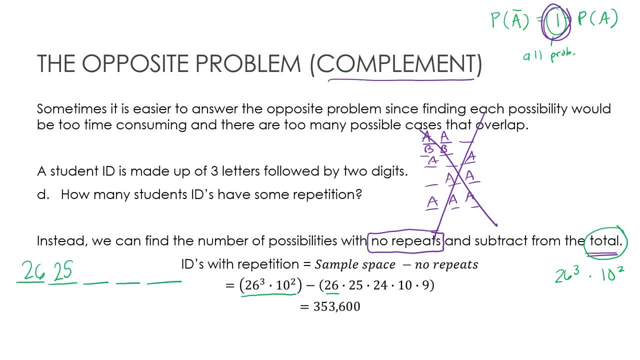 I can't repeat, so that's 25.. I can't repeat either of those, so that's 24.. And then again we have 10 for the first digit, but I can't repeat that digit, so there's nine. 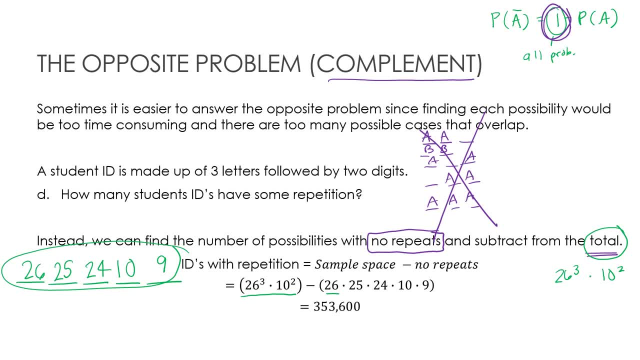 So, again, this was an answer to a previous problem that we did, as was this, And notice, now I'm just subtracting the two to find my total answer of 353,600.. So let's take a look at this last question. 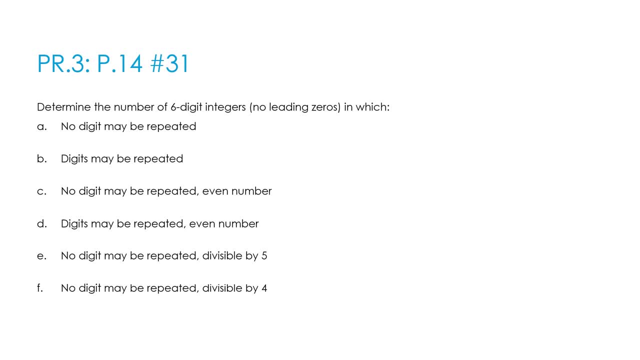 And some of these are pretty straightforward and some not so much, So what I would encourage you to do is to take your time on this, So it's very tempting to just not press pause and not try these questions on your own first, and I would discourage you from doing that. 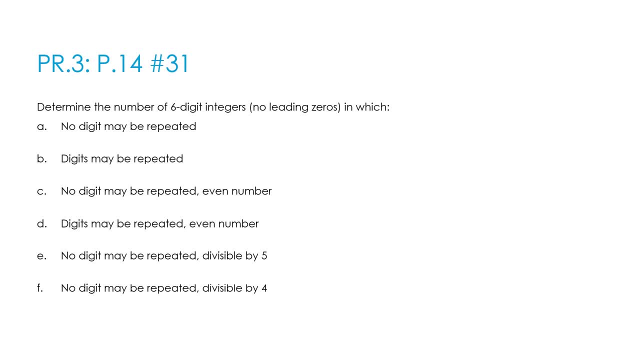 because as I go through them, you're going to say, oh yeah, sure, that makes perfect sense. But when you're actually trying these on your own, before you know the answer, you're going to have that moment of struggle where you're thinking: 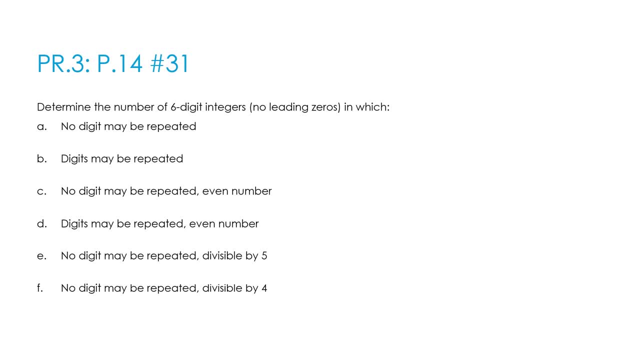 I don't know how to do that, And that's a very important moment because that's when you are learning how we can apply what we know. So press pause, try all six questions. When you're ready, press play to see how you did. 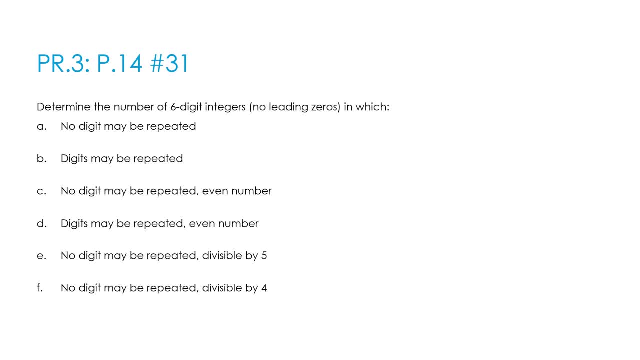 So before I started this question, I just started by looking at this. without even looking at A, B, C, D or F, I said I've got six numbers And I didn't look at any of the restrictions, except for it says no leading zeros. 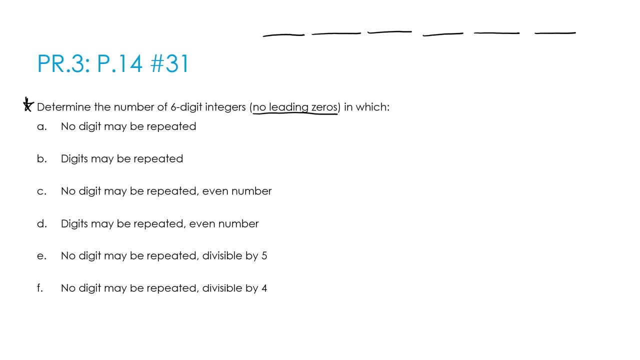 So I know that the digits include the numbers zero through nine. So the first digit can be not zero through nine because it can't be a leading zero. So my first digit could be one through nine, But any of the rest of my digits can be zero through nine. 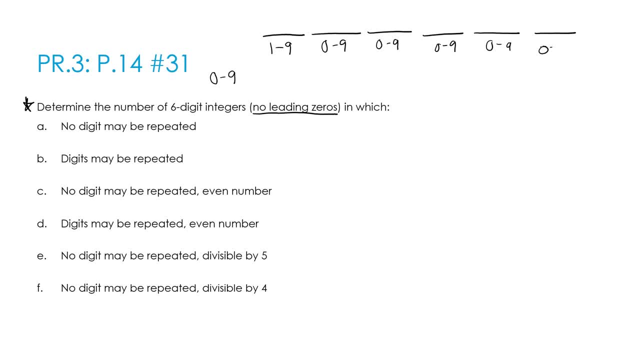 So how many options is that? Well, I know zero through nine is ten options And obviously one through nine is nine options. So that's a really good starting point. I have an idea of what the question is all about before I actually am trying to answer anything. 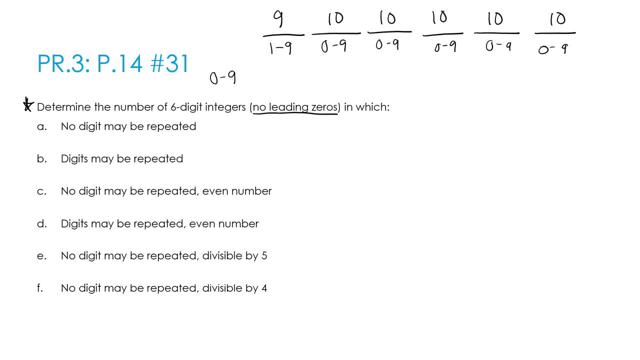 So now let's try to answer the first question. It says no digit may be repeated. All right, so let's use kind of what I came up with at the beginning and change it a little bit. My first digit: still nine options, because I can use any digit that I want except for zero. 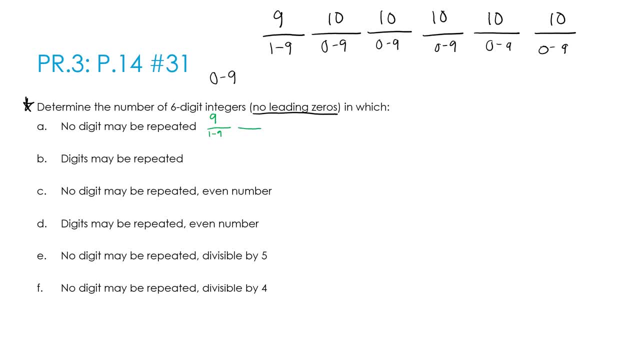 One through nine. This guy can be any digit except for whatever I put here. So there are still nine options, because I can use zero now, but I can't use whatever the first digit is. For my next option, I can use anything except for what either of these two are. 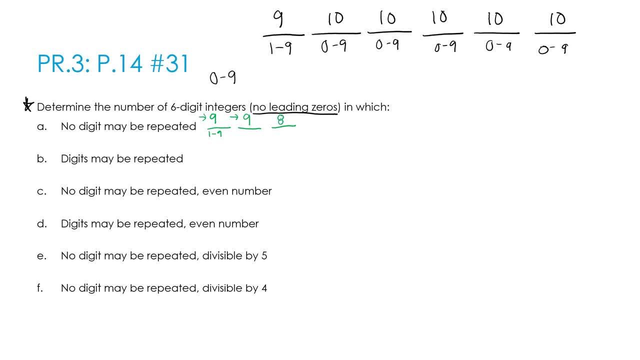 which means now I only have eight digits left because I've used two, And then I have seven digits left and six digits left and five digits left. So that's what I'm looking at, for A No digit may be repeated Nine times, nine times, eight times, seven times, six times five. 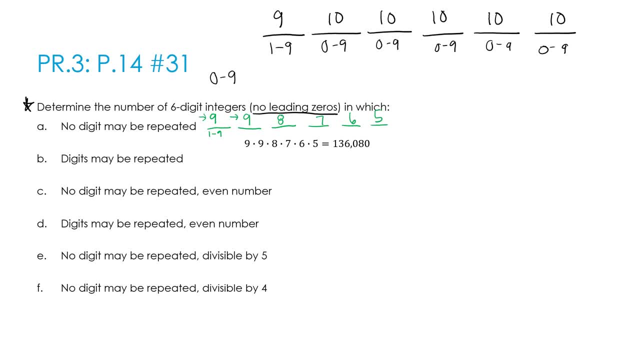 For B digits may be repeated. Well, good news. I already determined that one right up here. If I can repeat digits, that's what I came up with at the beginning, for the total sample space is nine times ten to the fifth. 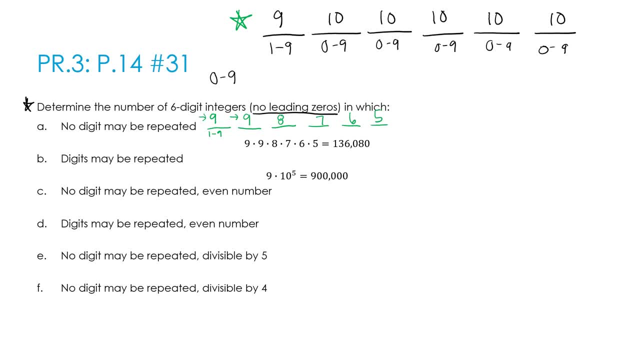 So now that we've done the easier ones, let's take a look at the ones that may hurt your brain a little bit. This one says no digit may be repeated and it's an even number. So we're kind of looking at this one. 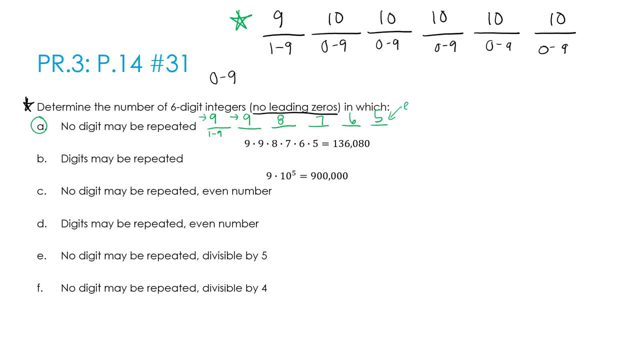 but we're saying: this guy has to be even. So you might be thinking: well, that works, because there's five even numbers, So let's just go with it. Okay, that's not going to work. Here's why I have this restriction, right here. 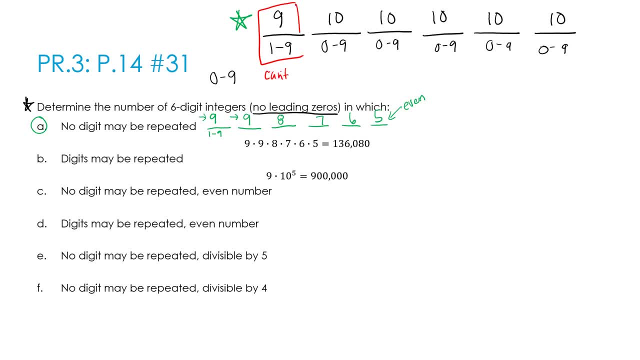 that says this guy can't be zero, which means when I have an even number, which is a number that would end in zero or two, or four, or six or eight, making it even, this guy is going to come into play because the first one can't be a zero. 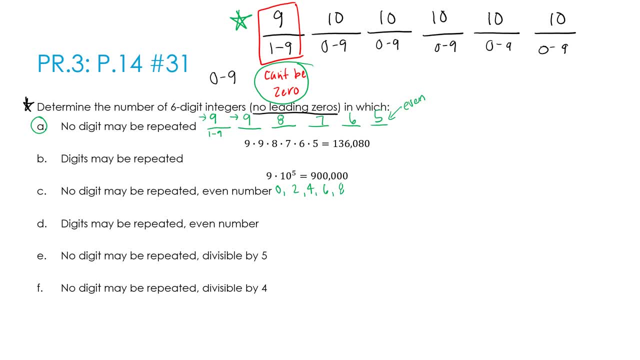 and that's going to change some of my possibilities. So what I have to do is actually think of two cases. So let's look at these two cases. If it ends in a zero, then I've got my nine options at the beginning. 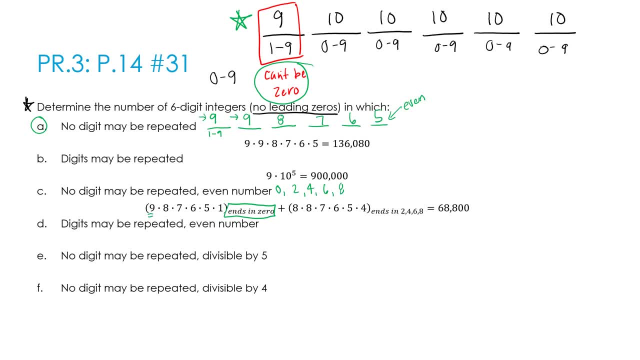 which is anything except for zero, then anything except for zero and whatever is here, and then anything except for zero and whatever is here and here, And same pattern. And then this guy: there's only one option, because that is a zero. So that's my first possibility. 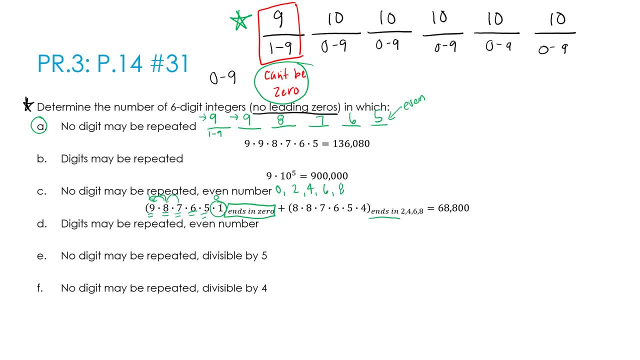 My second possibility is that it doesn't end in a zero and ends in one of my other, even numbers. So that's four options. So this guy can be anything except for zero and except for whatever this is. So I've kind of started at the end. 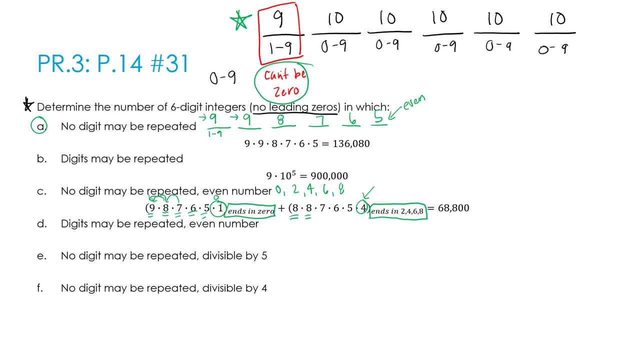 This guy can be anything except for whatever this is and whatever this is. So there's eight options. This guy can be anything except for those we've already assigned. Same here, same here. Of course, it's decreasing by one, because each time we assign one more. 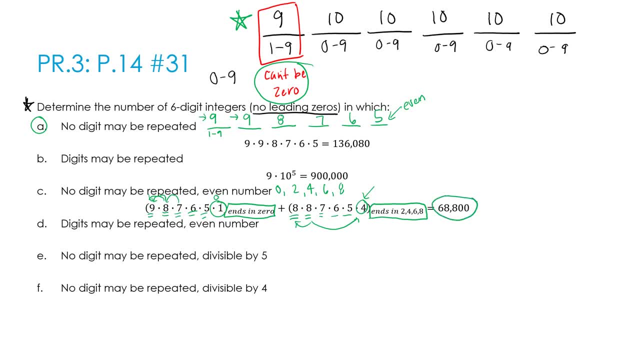 So then I show that work and show that then I'm finding the sum of those two possibilities. So whenever I break them into cases, that's a rule of sum. But then of course I was using rule of product to find the probabilities of each case. 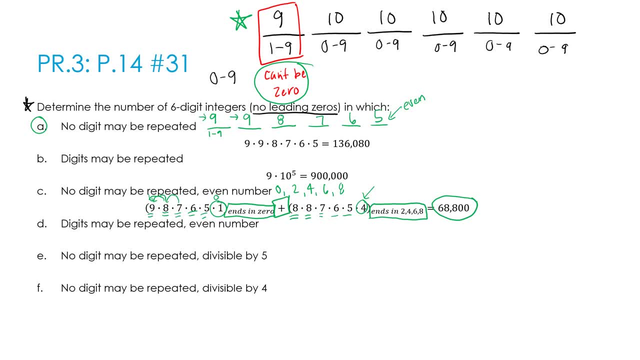 So if, at this point, you'd like to press pause again and try D, E and F again, if you didn't get them the first time, that would maybe be a good idea. Otherwise, we're going to forge ahead. Here we have. digits may be repeated. 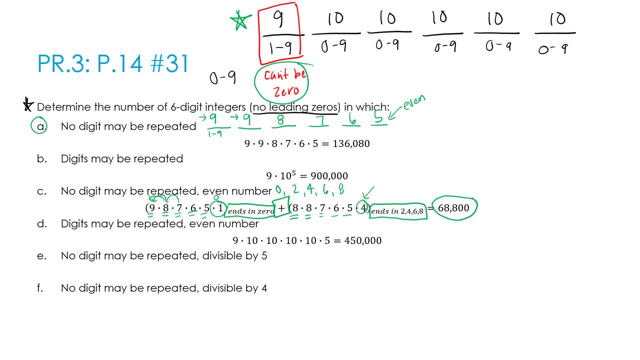 and it's an even number. So this one's much more straightforward, because I've got five different options here For ending in an even number: zero, two, four, six or eight, And it's okay if we repeat things. The only restriction, of course. 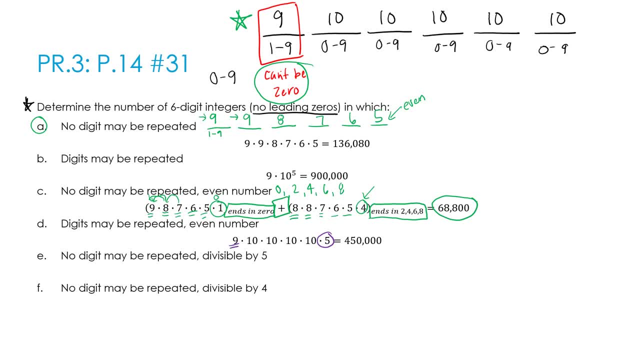 is that nine at the beginning, because I can't use a zero. So D is pretty straightforward. For E, no digit may be repeated divisible by five. So if it's divisible by five, what is my number going to end in? It's going to end in a zero or a five. 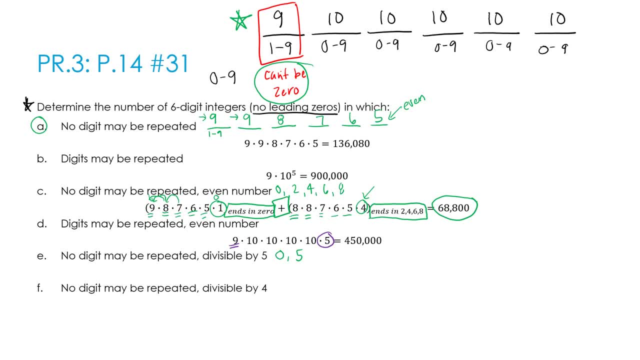 Well, as you can see, that's going to bring me back to a question like this where I'm going to have cases because I've got that restriction with zero, So really I'm going to have the case where it ends in a zero. 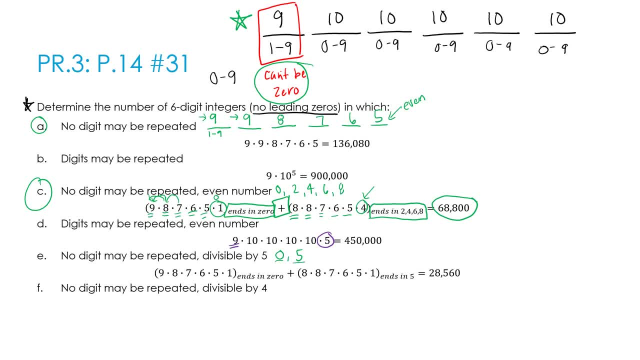 and the case where it ends in a five, And here's what that looks like. If it ends in a zero, I have one option for the end. I have nine options here. everything except zero, then eight, seven, six, five. 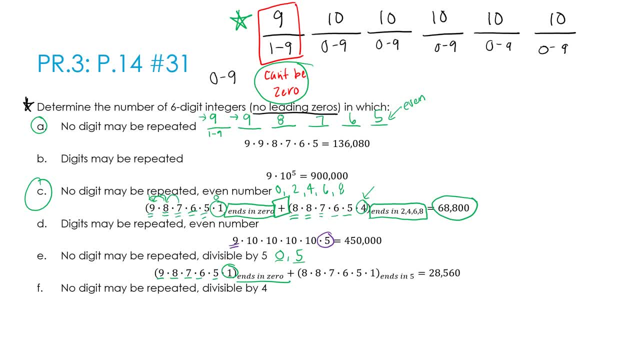 So basically the same pattern we used before. If it ends in a five, again one option here. Here I have eight options. Why? Because it can't be five and it also can't be zero, So that's why there's only eight. 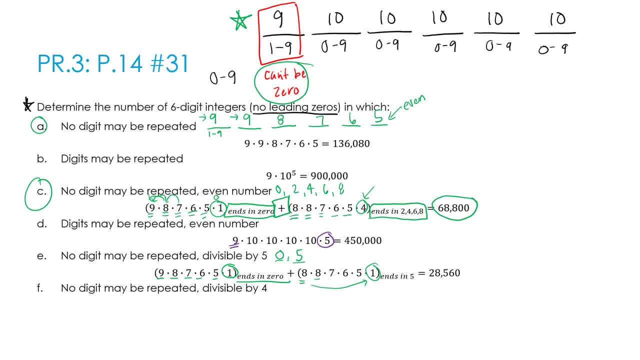 instead of nine options, And then eight here, because it can't be a five and it can't be whatever I used here, And then it continues to decrease from there, So that total sum 28,560.. And last one, this one's a real bear. 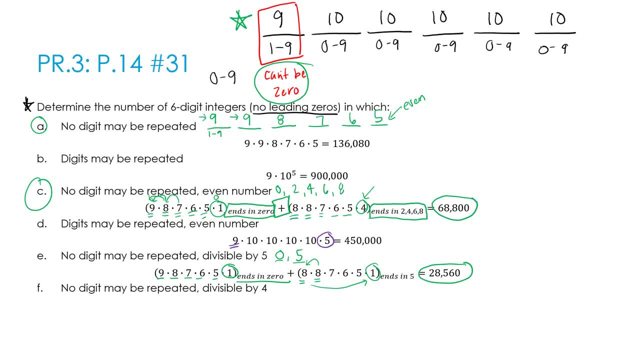 So if you got this one, congratulations. This one says no digit may be repeated and divisible by four. The difficult thing here is that if it's divisible by four, I can't just say that it ends in two, four, six, eight or zero. 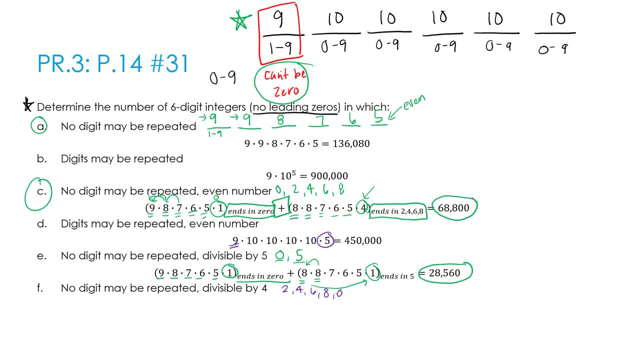 because that just makes it even. And of course there are even numbers like two and six and 10 that are not divisible by four. So I have to take this guy to the next level. I have to think about numbers that are divisible by four. 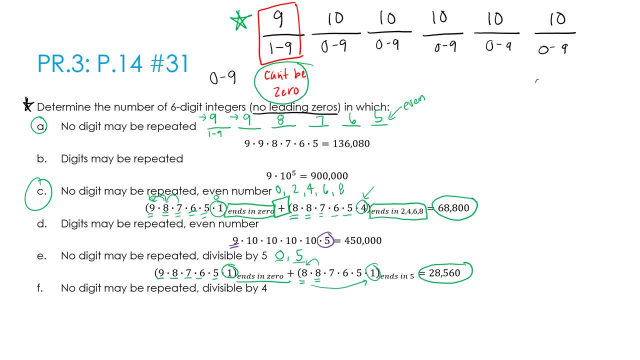 which are two digits. So I would start thinking about zero four, zero eight, one two being the last two numbers, one six being the last two numbers, et cetera, et cetera, et cetera. 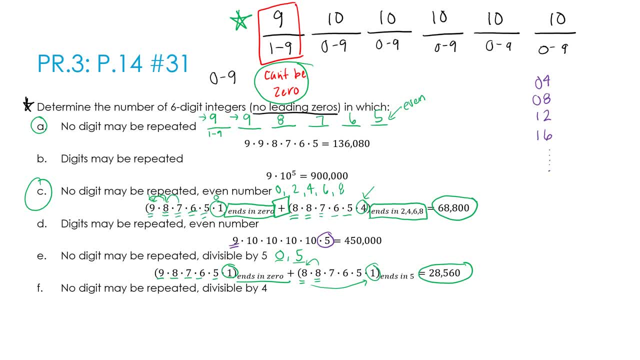 Why would I do that? Because I need to know what all of the options are. And then I have to go back to what I learned here, and here I have to think about my zeros. So let's take a look. We looked at two digits being divisible by four. 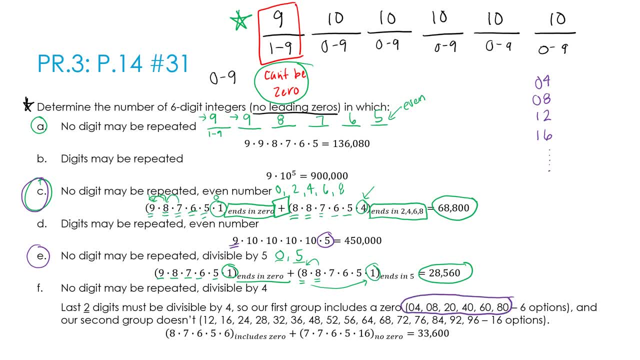 And notice. what I've done is I've broken them into a group that includes a zero and a group that does not include a zero, because, again, I'm looking at my two different cases. So my first case includes a zero and that means there are the six options. 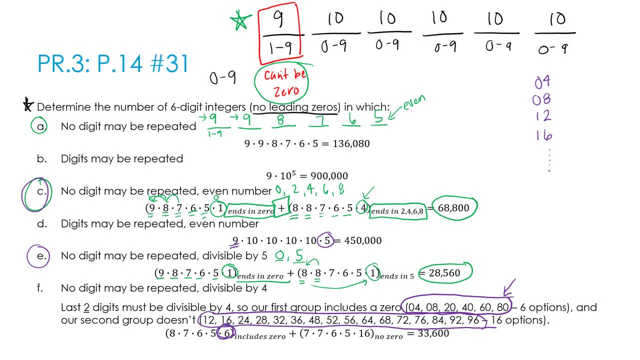 And remember I only have two digits, So I'm only going to be multiplying five items instead of six. Then this guy starts with eight options- Only eight, because I already have the zero here- and then whatever number other than that I used, So there's eight left. 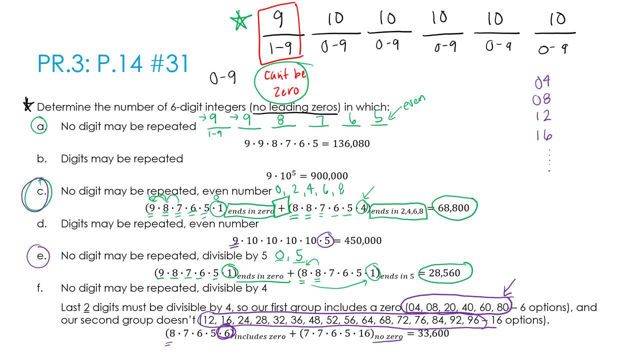 and then it decreases from there. Four does not end in a zero. There's all of these guys. There are seven options here, because it can't be a zero and it can't be either of the numbers used here. But then seven for the next option. 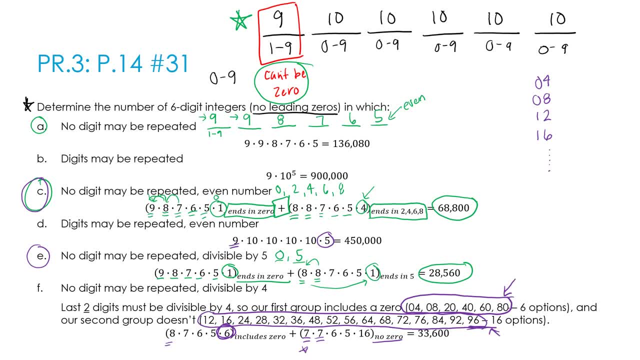 because it can't be this guy or these guys, but it can be zero, and then it decreases from there, and then 16 for the last two. Adding those together, I get my final solution of 33,600.. Good work.